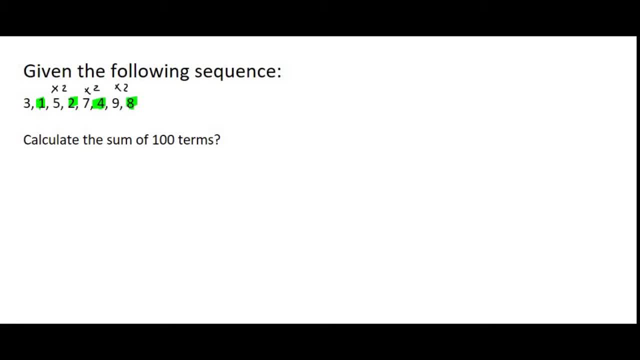 one to two, you times by two, and then to four, and then to eight. So we have a combination question over here where we have half of the terms being geometric and the other half arithmetic, So it's super easy to calculate. We'll take 50 terms using an arithmetic pattern. 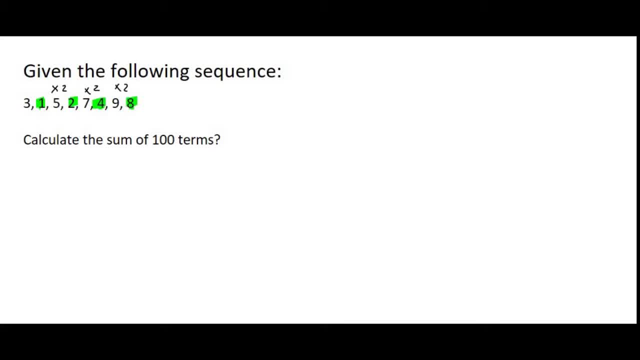 and the other 50 terms will be the geometric. At the end we'll just add the two answers together and that'll be the sum of a hundred terms. So we know that the sum of an arithmetic pattern can be calculated with the following formula: And so let's see what we get. So we know that. 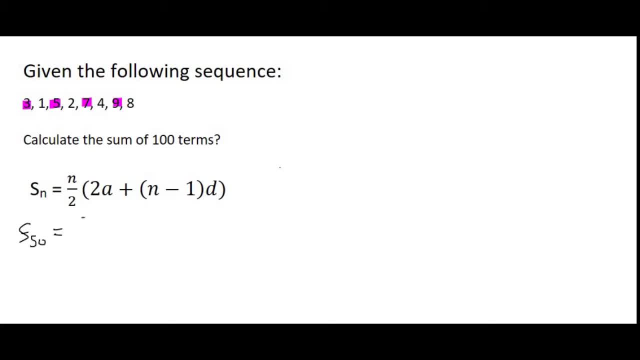 the sum. well, that's going to be for 50 terms- is going to be 50 over 2.. So 50 terms, because half of the terms are going to be arithmetic and half will be geometric. We'll then say two times a. Now, a is usually term one, which in this case will be three plus n is going to be 50 minus one. 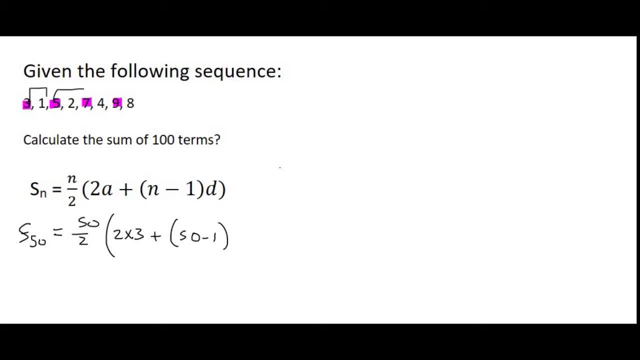 And the common difference between those numbers for the arithmetic is two. You can go ahead and type all of that in on the calculator and we should get an answer of 2,600.. Now we can do the other half of our sequence, which is a geometric, So we use the sum of a geometric. 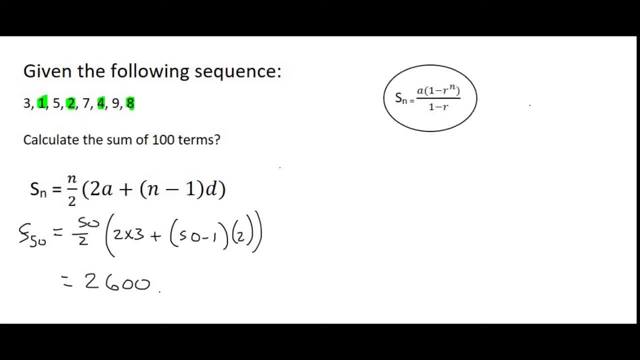 pattern which is given with this formula over here, And so we'll find the sum of 50 terms, And so a is not going to be three. A is going to be one because we're looking at the geometric pattern. specifically, R is the number that you have to multiply with to get to the next term. 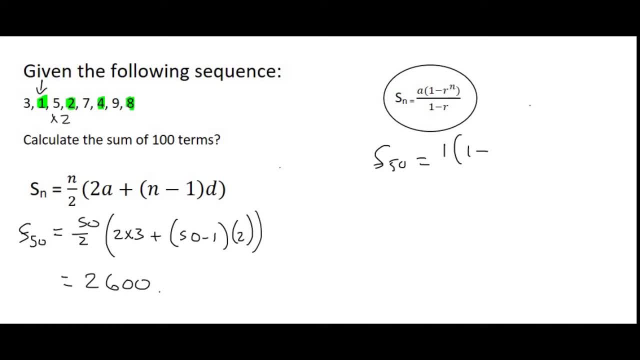 And that's going to be two, because you're saying one times two to get to two, and then two times two gets you to four, and then four times two gets us to eight. So R is going to be two and then we'll have 50 terms for that pattern. 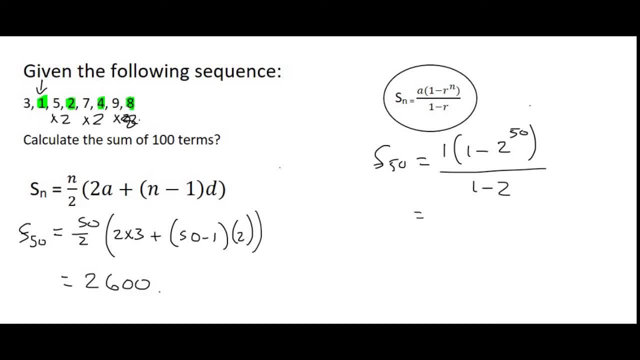 And then we'll say one minus two at the bottom And then you can just put all that, all of that, on the calculator and that will give us a value of. that actually gives us a huge number, And I should have chosen a smaller number of terms, because that two to the power of 50 is an extremely big. 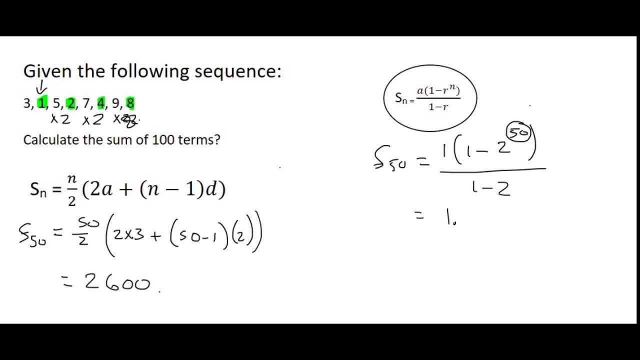 number. So it's a bit of a silly example now, because you'll see what's going to happen. But if we round to two decimal places, it's going to be approximately 1.13 times 10 to the 15.. And then we said that we simply have to take these two numbers and add them together. 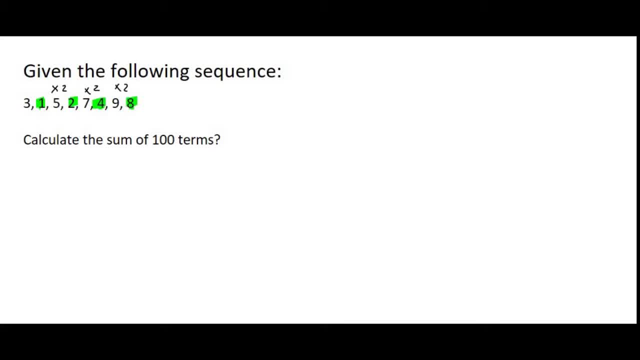 and the other 50 terms will be the geometric. At the end we'll just add the two answers together and that'll be the sum of a hundred terms. So we know that the sum of an arithmetic pattern can be calculated with the following formula: And so let's see what we get. So we know that. 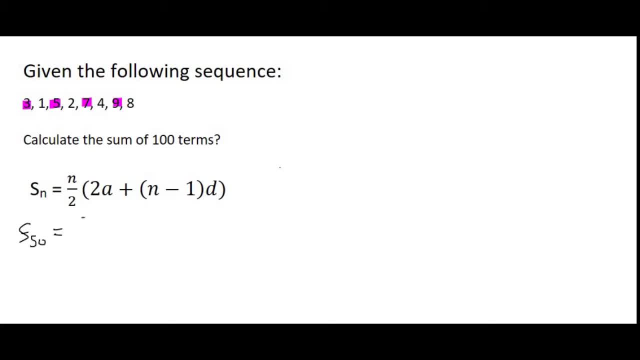 the sum. well, that's going to be for 50 terms- is going to be 50 over 2.. So 50 terms, because half of the terms are going to be arithmetic and half will be geometric. We'll then say two times a. Now, a is usually term one, which in this case will be three plus n is going to be 50 minus one. 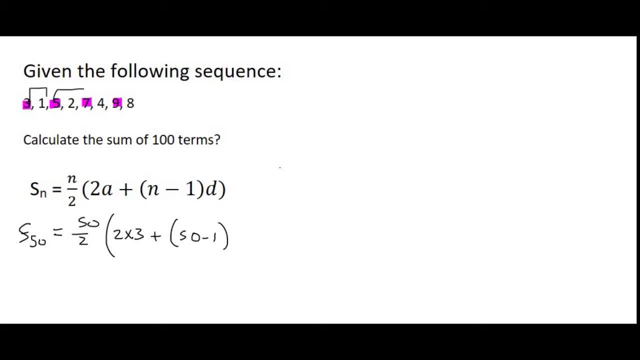 And the common difference between those numbers for the arithmetic is two. You can go ahead and type all of that in on the calculator and we should get an answer of 2,600.. Now we can do the other half of our sequence, which is a geometric, So we use the sum of a geometric. 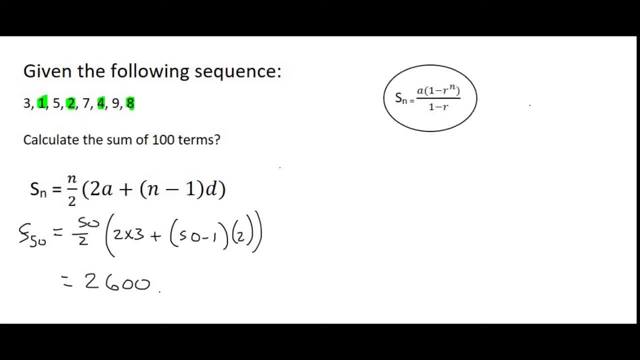 pattern which is given with this formula over here, And so we'll find the sum of 50 terms, And so a is not going to be three. A is going to be one because we're looking at the geometric pattern. specifically, R is the number that you have to multiply with to get to the next term. 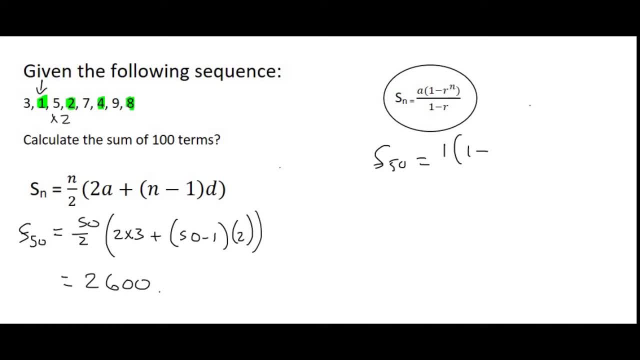 And that's going to be two, because you're saying one times two to get to two, and then two times two gets you to four, and then four times two gets us to eight. So R is going to be two and then we'll have 50 terms for that pattern. 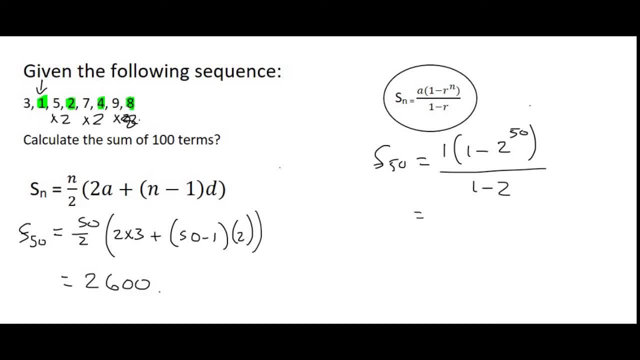 And then we'll say one minus two at the bottom And then you can just put all that, all of that, on the calculator and that will give us a value of. that actually gives us a huge number, And I should have chosen a smaller number of terms, because that two to the power of 50 is an extremely big. 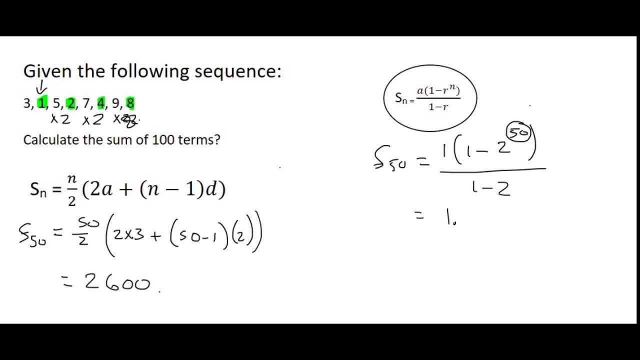 number. So it's a bit of a silly example now, because you'll see what's going to happen. But if we round to two decimal places, it's going to be approximately 1.13 times 10 to the 15.. And then we said that we simply have to take these two numbers and add them together. 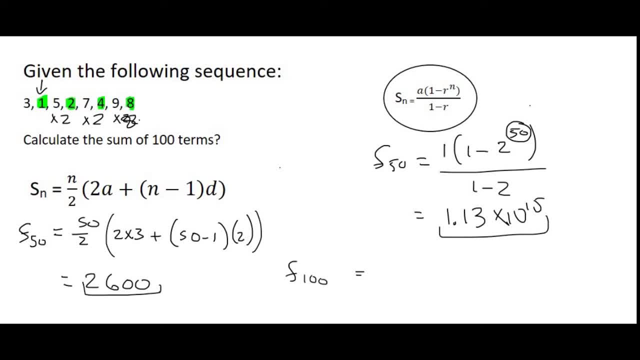 But if we do that, we're still going to get a, so that some of the 100 terms is still going to stay. 1.13 times 10 to the 15. Why? Because 2600 is so small compared to this huge number. This is a.